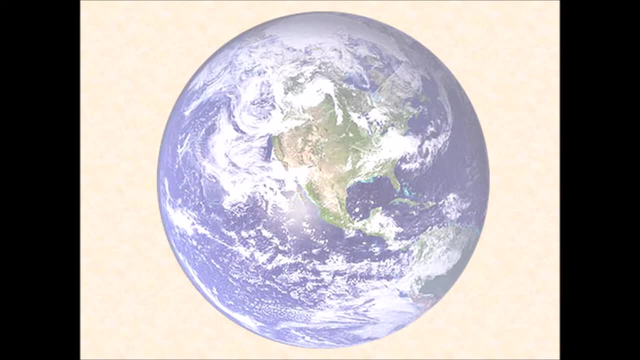 concept in more detail. So if you're working on the worksheets, you have got a box with the Earth in the middle and we're going to turn this into a diagram of global atmospheric circulation. If you're not working on the worksheets, you can easily do this on a plane. 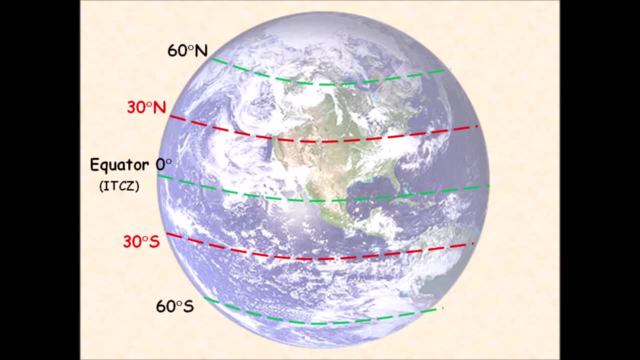 a flight or a plane that's in the middle of the Earth. So if you're working on the worksheets piece of paper, So we're going to start off and we're going to add in our lines of latitude, So we've got the equator at zero degrees, which we can also call the intertropical convergence zone. 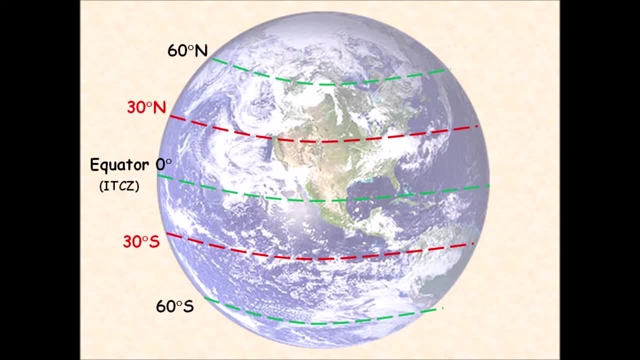 so I-T-C-Z for short. Then we've got to put 30 degrees north and 30 degrees south latitude lines on our planet as well, as well as 60 degrees north and 60 degrees south. Now, when it comes to global atmospheric circulation, 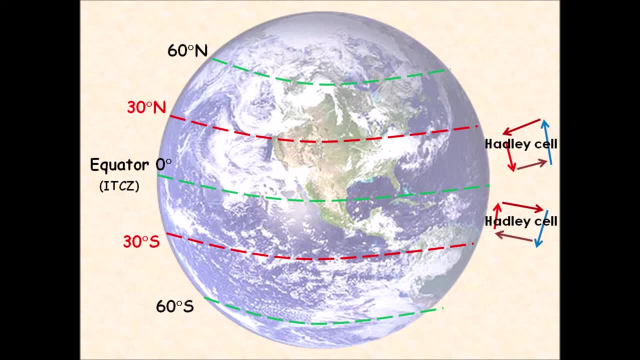 there are three main cells. You've got your Hadley cell and that's the first cell we're going to draw on the right-hand side of our planet. And the Hadley cell is where we have air moving between the equator and 30 degrees north and 30 degrees south. 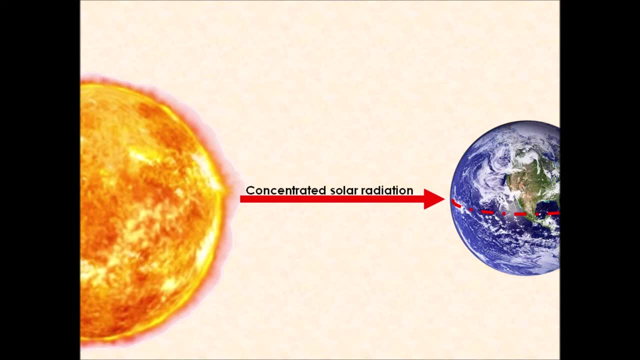 So what happens on the equator or the intertropical convergence zone is that the sun is sending the most concentrated amount of solar radiation towards the equator. So the sun heats up the earth at the equator the most and that heats up the air on the equator and the 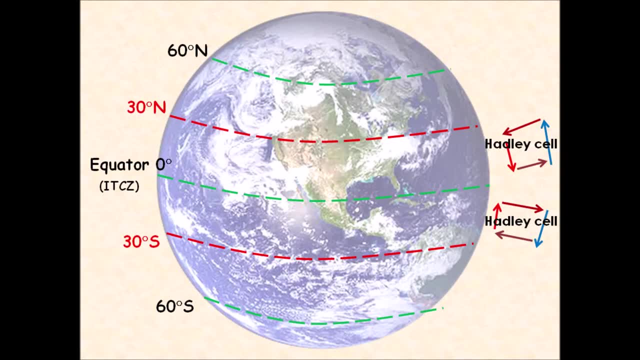 intertropical convergence zone. This causes the air to rise around the equator, creating an area of low pressure. So between our two Hadley cells we can add in that low pressure area. This low pressure air is rising air, which is why, if you notice your two arrows in your head, you're going to 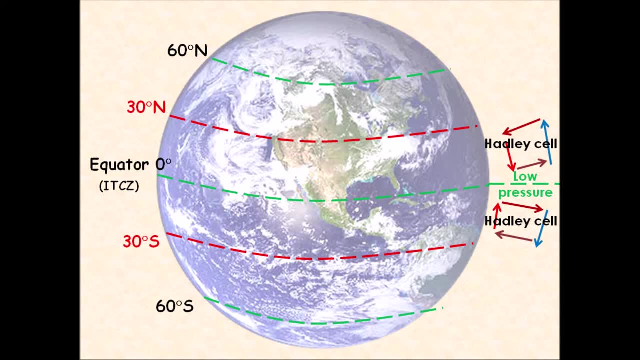 see the Hadley cell either side of the low pressure are rising, And this is because when we have low pressure, the air rises, cools and condenses and creates clouds, which then leads to precipitation or rainfall. Now, if we then think about the direction that air then is, 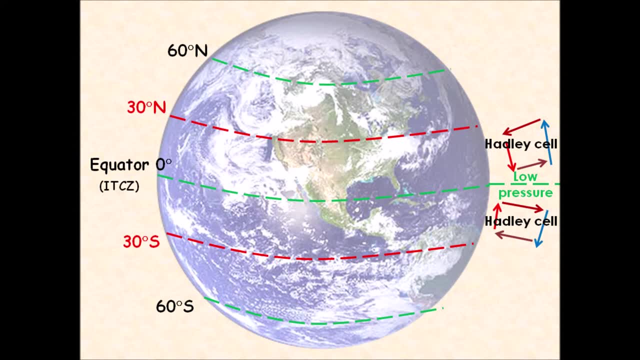 circulating to within our Hadley cell. So within our Hadley cell the air then moves to 30 degrees north and 30 degrees south of the equator And that then creates high pressure on those areas that 30 degrees north and 30 degrees south. And that is because the air 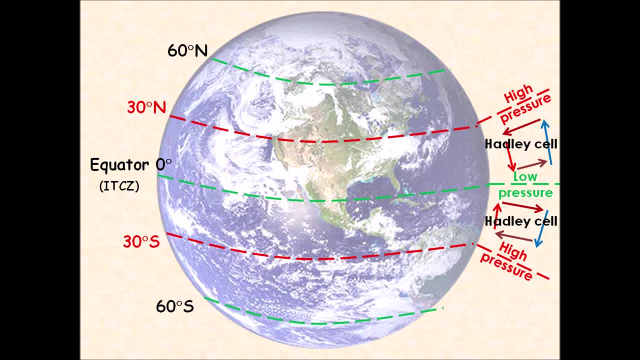 is sinking. So it's moving back to the equator in a circular motion. it's descending in that circular motion within the Hadley cell And the process obviously repeats and occurs again. So the sun heats up the air at the equator, it rises to cause low pressure and then it descends at 30 degrees. 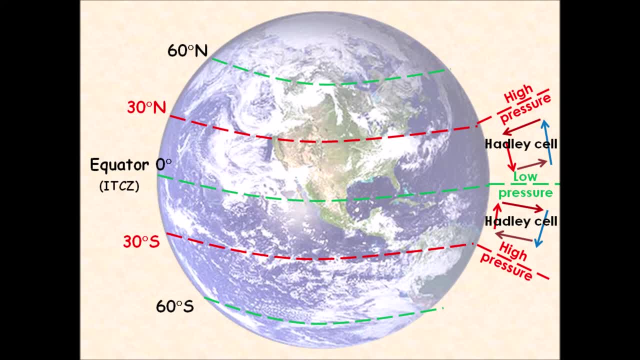 north and 30 degrees south, And that causes high pressure there. The high pressure will instead create clear skies and dry conditions, because we have not got any evaporation taking place there to create clouds. Now, this is where we then introduce our second cell, which is known as a, our ferrule cell. And our ferrule cell is when 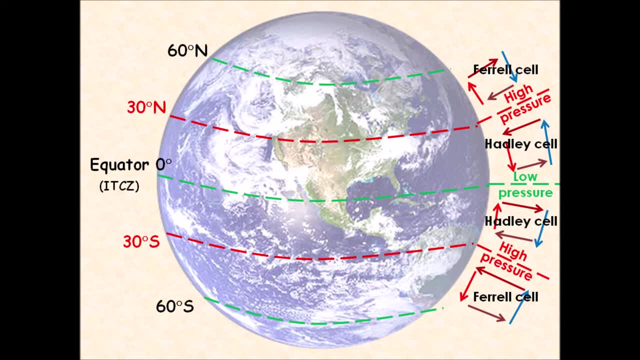 we have the circulation of air moving now between 30 degrees north and south- our planet- and 60 degrees north and south, So again at 30 degrees north and 30 degrees south. the air has sunk, it's descended to create that high pressure and it will either move back to 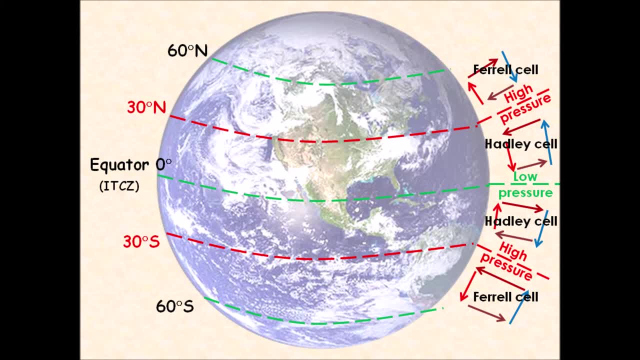 the equator or within our ferrule cell. now it will move 60 degrees north or south. So when it is then included in your ferrule cell and comes into contact with the latitude lines of 60 degrees north and 60 degrees south on our planet, the air again will rise and create that area of low. 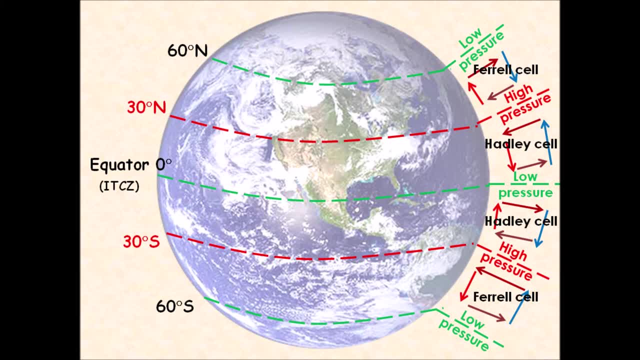 pressure So that rising air again will cool and condense to create clouds and therefore lead to precipitation. So between your Hadley cell and your ferrule cell you have areas of high pressure because that air is descending, it's coming down, but between your ferrule cell and your polar cell 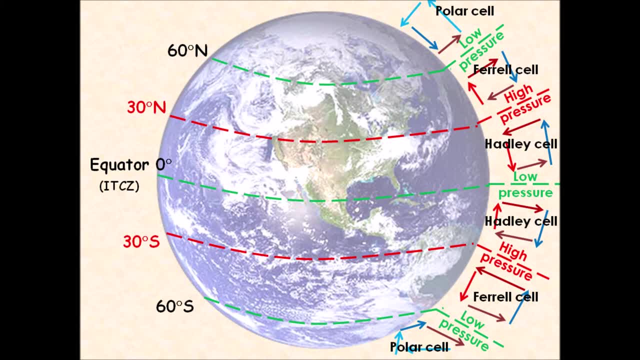 you have that air rising again to create that low pressure. So, when it comes to the equator, you have that air rising again to create those areas of low pressure. Now, that then leads us nicely on to our third and final convection cell, which is known as the polar cell, and these 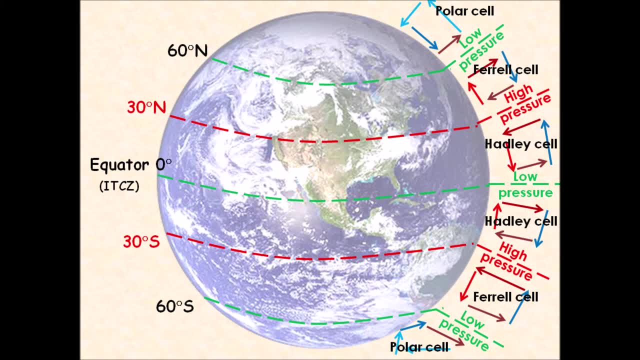 particular cells will move air between the 60 degrees north and south latitude lines and the north and south poles. At the north and south poles the air again is sinking, causing an area of high pressure. So remember, high pressure is when the air is down and the air is up. So when it comes to